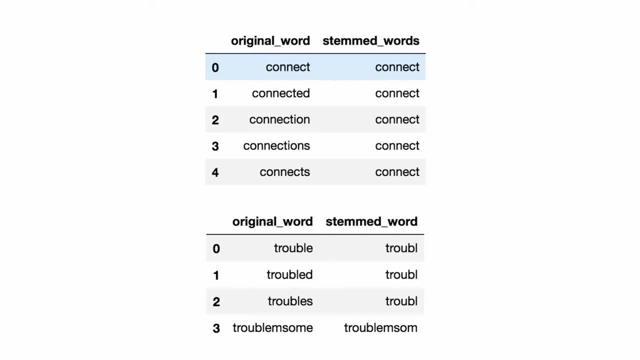 Hi guys, what's up? Today we'll learn how to simplify words in NLP process. You'll get to know lemmatization and stemming technique. First let's describe the problem. Many words in English can take on several forms. For example, verb go may appear in the third. 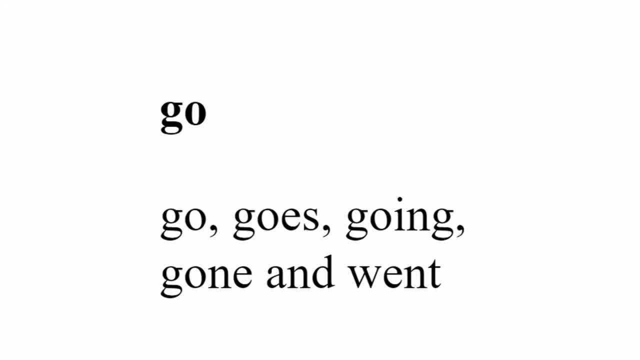 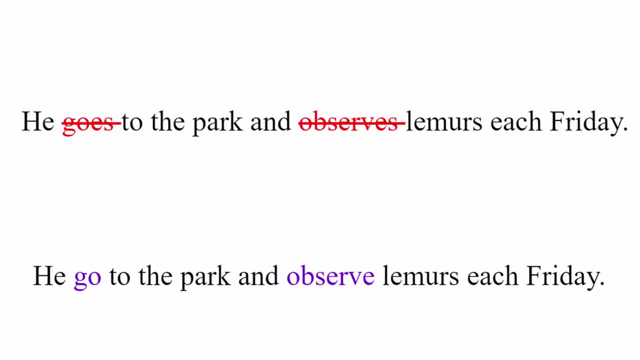 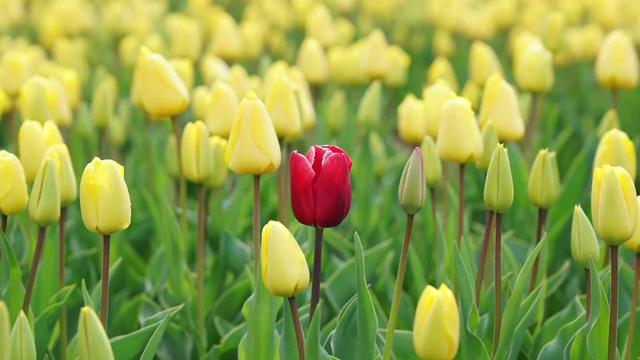 person as goes. It turns out that NLP models often work better when generalization is present, which means that in this case, we would go back to the basic form go instead of using goes in further research, Each problem is unique, so before moving words, 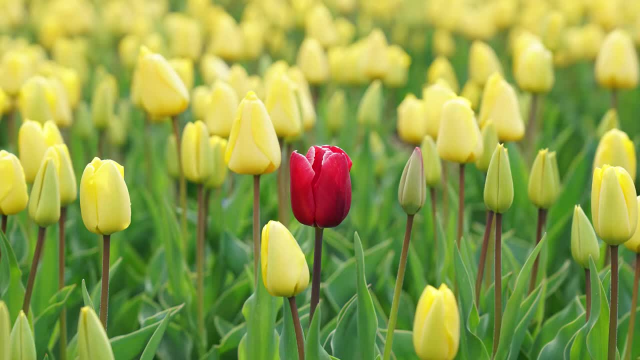 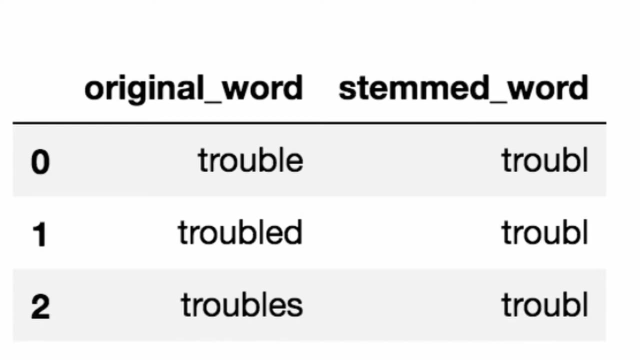 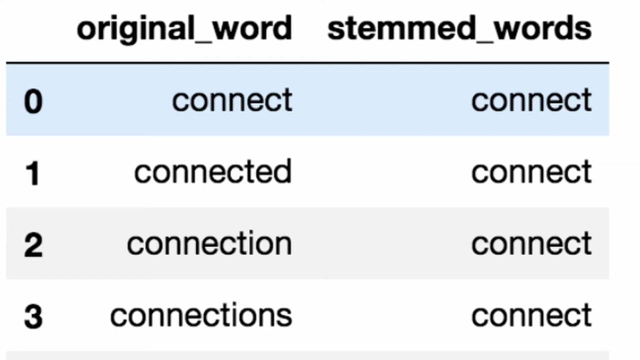 back to its root form, you should analyze whether it is beneficial for your case. You may check if some essential information is lost during the process or if only irrelevant information is gone. When you know that you need a basic form of the words, then you may apply some method to achieve it. 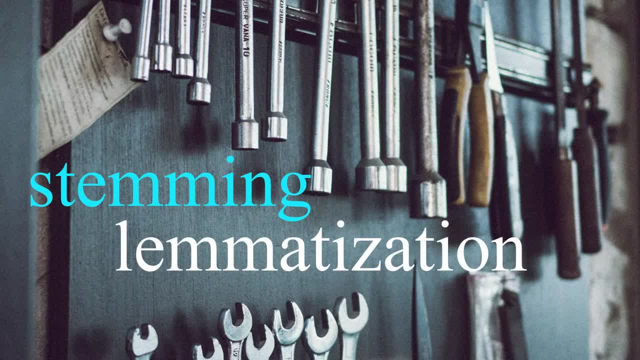 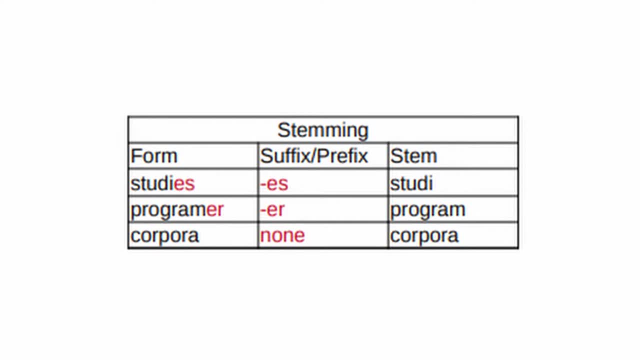 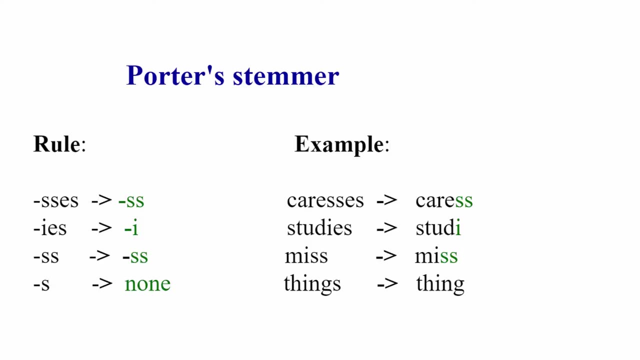 You may encounter two techniques: stemming and lemmatization. Stemming algorithms work by cutting off either the end or the beginning of the word. How is it able to do it? It's just referring to a list of common prefixes and suffixes that are present in a given word. However, some words may seem to have suffixes. 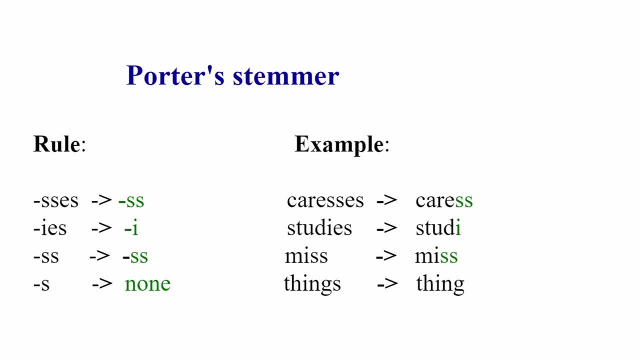 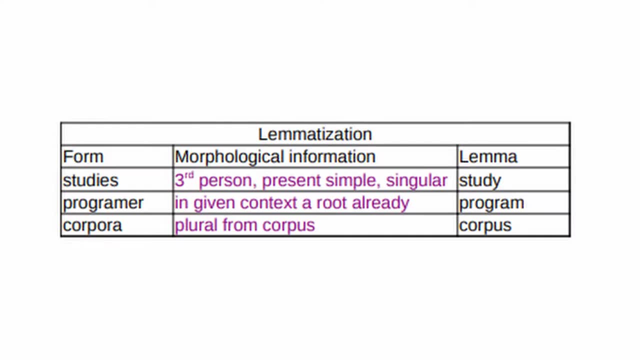 but in reality they are just constructed in this way. This means that stemming methods may often misidentify the part that should be removed. On the other hand, lemmatization is the process of converting a word to its base form with the intention to find the 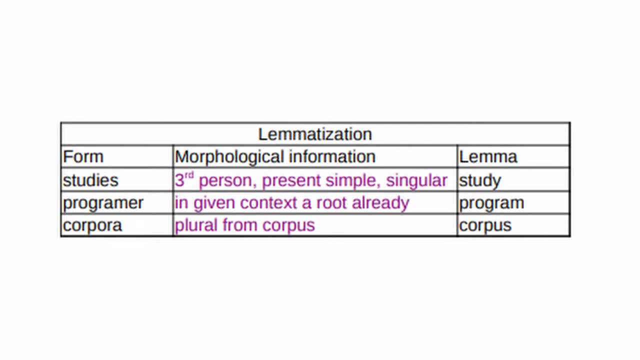 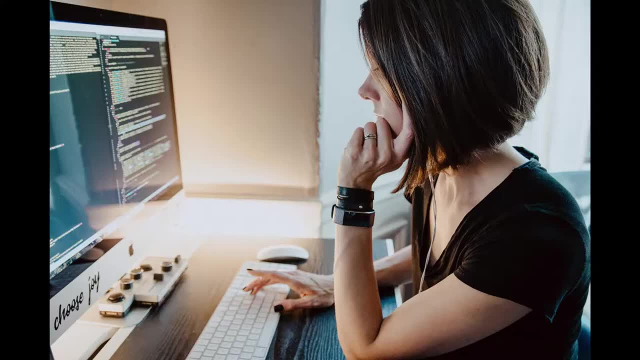 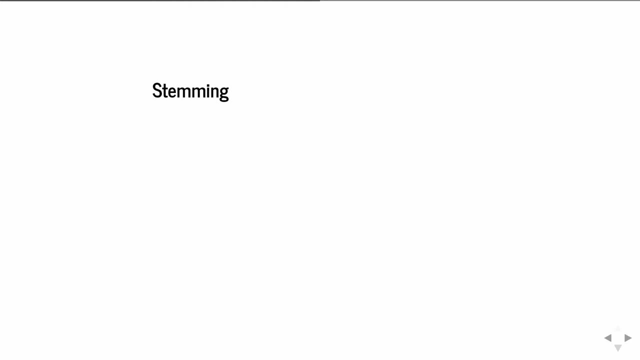 root of the word. This means that it tries to take into account the context in which the word appears, instead of using only predefined suffixes or prefixes. Let's see how to apply in Python both of these techniques. To apply stemming, we may import necessary methods from an ltk library. 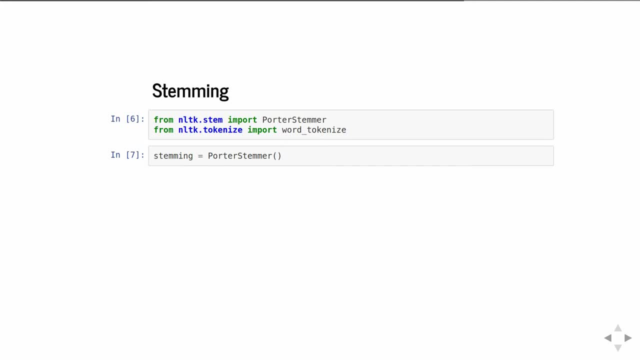 Then we define our stemming variable. Here are the words that will be used. as examples, We will use the same method to compare the results from stemming and lemmatization. With the usage of loop, we may see how the words were being transformed.